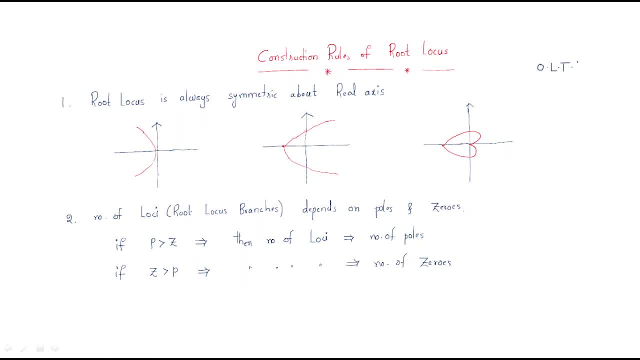 this open loop transfer function. open loop transfer function. we are discussing about the closed loop poles, but we will use by the open loop transfer function. in this we will discuss. it has some construction tools. the first rule is: root locus is always symmetric about the real axis. the most important point is it is only symmetric about the real axis. it's the path. 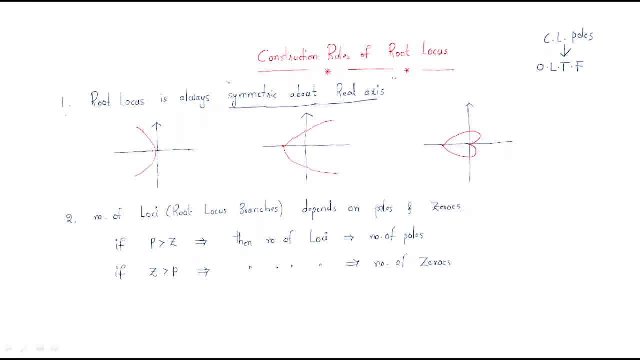 consisting of the symmetric of the real axis. look at here. this is the s plane and it is the axis: real axis negative side and real axis positive side. this is the positive real axis. this is the negative real axis. the construction root locus is the represented by the red, red ink. so 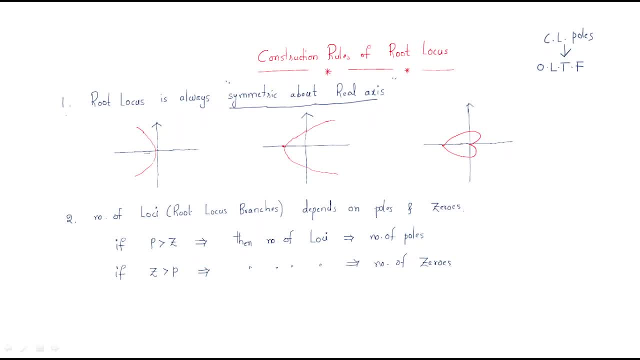 so this is the root locus here. also, it's look like symmetric about the real axis in the second session. this is the red line, this is also the symmetric about the real axis and this is the. it is also the symmetric about the real axis, so it's look like a symmetric about the real axis. 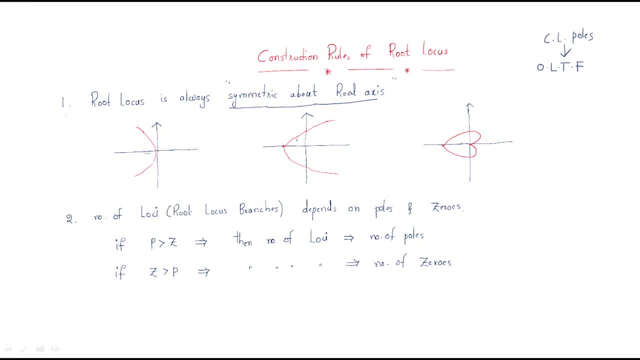 that's why, the most important point, if you take the any root locus, that root locus is always symmetric about the real axis. that means the path is always around the real axis right. the second point: number of lucy. generally, in short form, root locus will be called as the lucy. 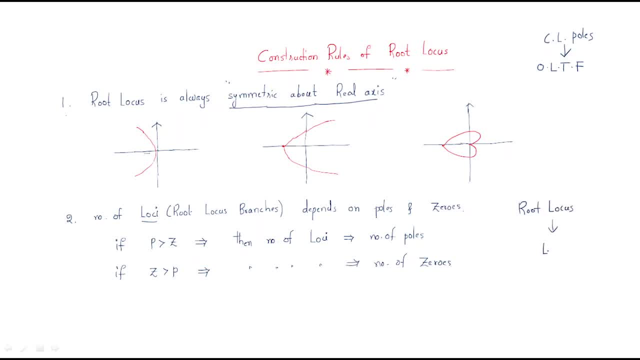 so we are going to start discussing root locus. so what called crux volume we can consider as a fare volume. so family, we be a family in limits, we be a unit in Sarawak. okay, so number of poles will be decides. when poles is greater than zero, the number of root locus will. 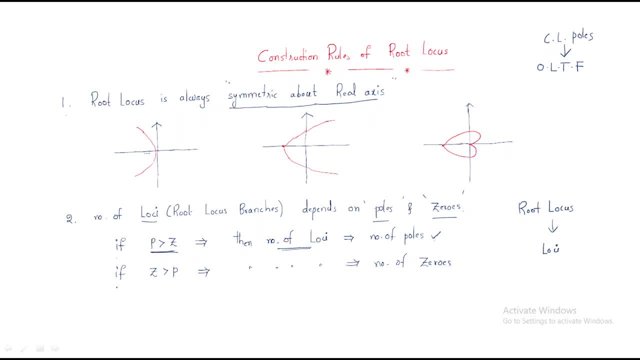 be equal to number of poles. second, if zeros are greater than poles, in the given equation zeros is more than the poles. then number of root loci: equal number of zeros. so bigger part will decide the number of root locus. number of root locus will be bigger part. that will depend on the 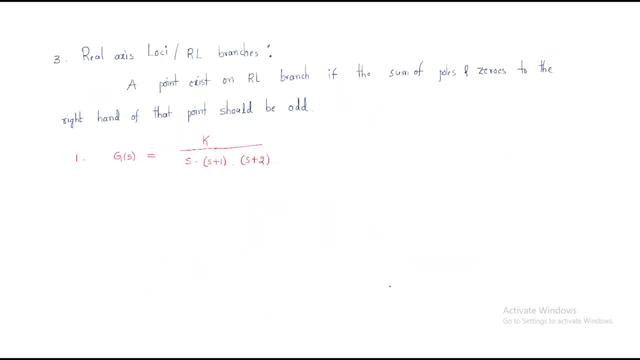 poles and the zeros. next point: the real axis loci. that means real axis loci are root locus. both are same branches. so how many real axis root locus branches? how will be decided? that will be look at here. a point exists on the rl branch. a point exists 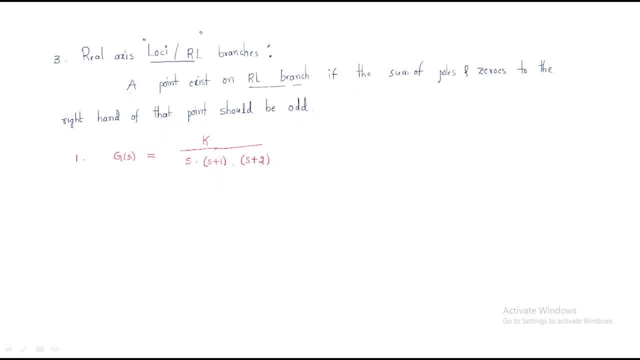 on the rl branch. if sum of poles and zeros to the right hand of that point should be odd, right hand that point should be add, okay, odd, then the root locus is possible. so to understand this statement, just solve one problem. look at here we have a one problem. 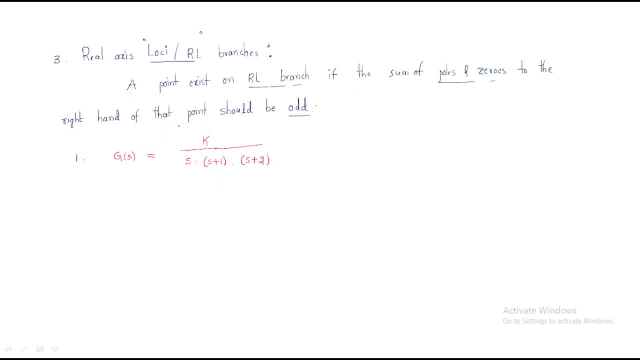 then we will find out to understand this concept. so here, given open loop transfer function g of s equal to k by s into s plus 1, s plus 2.. here we have the poles, only we have the poles, that is s equal to 0, and second pole is s equal to minus 1, and third pole: 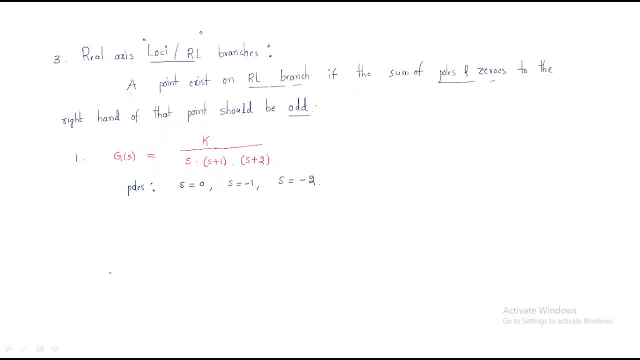 is s equal to minus 2. okay, we don't know where is the root locus diagram, so for that purpose, i am drawing the s plane. so this is the s plane. this is the s plane generally. so in this s plane, we have the poles. we have the poles. that is one s equal. 0 is the one flow, one pole. this is s equal. 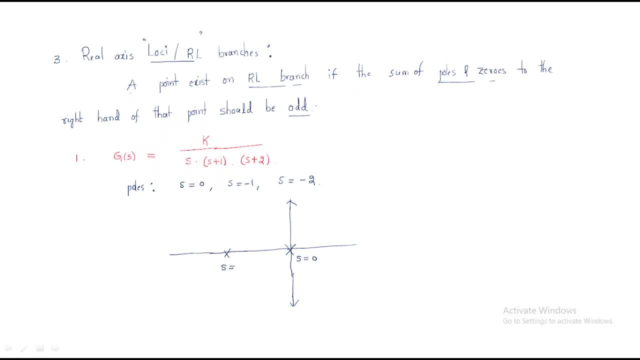 0 is the one pole and s equal to minus 1 is the another pole and next s equal minus 2 is the another pole we have. and these are poles, just at this point. look at this point, this point, right side. add the number of poles and zeros. is there any number of poles and zero at this point? 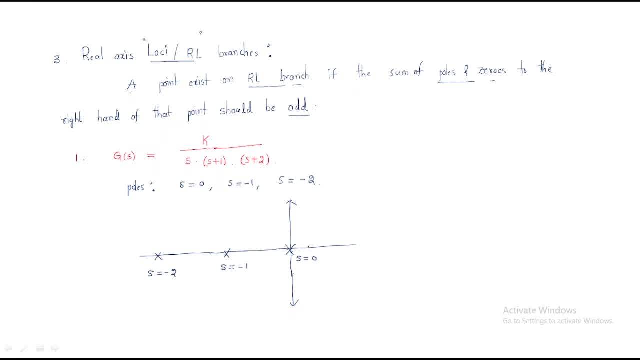 these points are 0 poles and zeros, so it doesn't have any root locus. but at this point, right side, the summation of poles and zeros is one. summation of poles and zeroes is one. so that's why we have one root locus branch here. that's why we have the root locus branch is here, so that root locus branch will be represents. 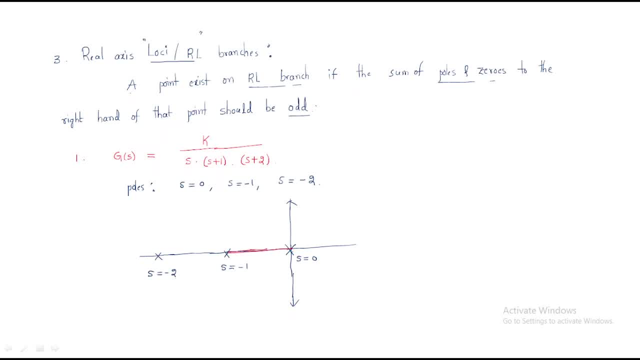 with like this. so we don't know, but we have the root locus branch between s equal 0 and s equal minus 1. okay, just here at this point we have right side 1 summation of poles and zeros. pole is 1, 0 is. 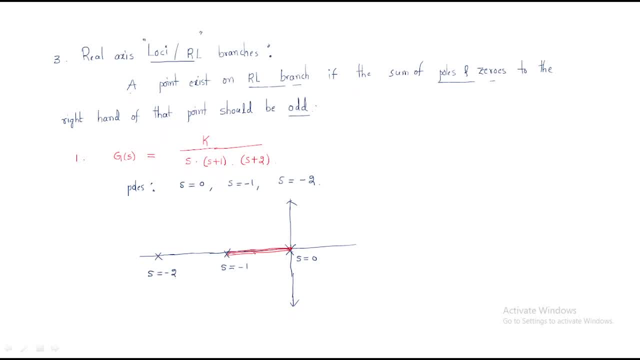 0. so then we have one root locus for this branch and at this point we have the summation of poles and zeros is 2 here. so that's why we don't have any. we don't have any root locus at this point. we don't have any root locus, okay, so always look at this at this point. look at the right side. 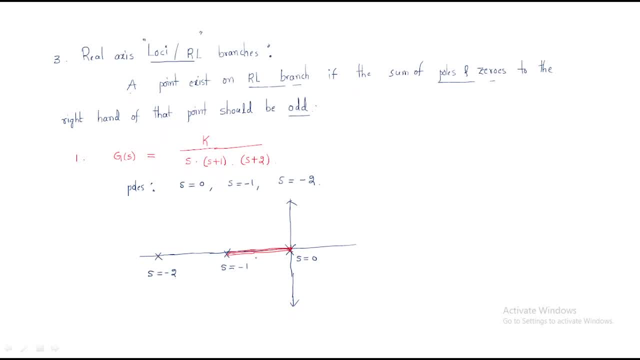 right hand side at this point, look at the right hand side. same here. at this point, look at the right hand side. they here, right hand side, we have one pole is there. that's why it has a root locus. at this right hand side. there is no poles and zero. that's why we 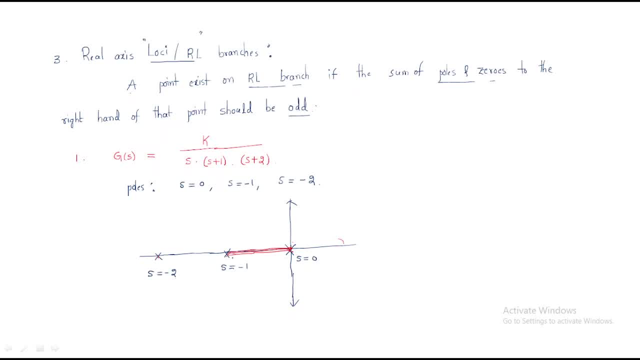 doesn't have any root locus at this side. we have one pole and one zero. that two poles is there. even number of poles is there. that's why we don't have any root locus here. we don't have any root locus here. okay, and so this is the process. okay, the next problem. look at the next problem. the problem is: 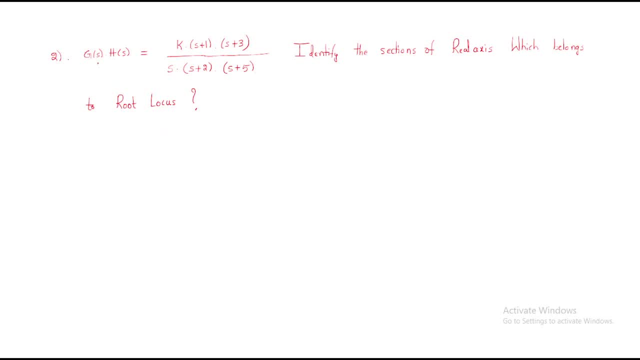 here the given system: j of s, h of s. so sometimes you will confuse why this h of s. so always keep in your mind, whenever the system is given like j of s and h of s, it is always a unity feedback system. keep in your mind, that is the unity feedback system. 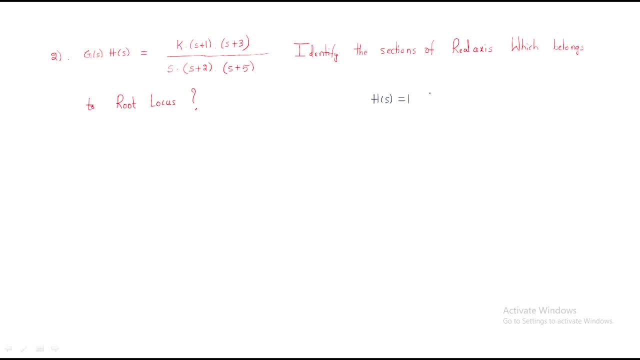 h of s and h of s are the same thing. so this is the process. okay, next problem. look at the next problem. j of s is equals to one, always. what is why? why it is one. it is unity feedback system. unity feedback system. that's why g of s and h of s means nothing, but simply j of s. both are same. 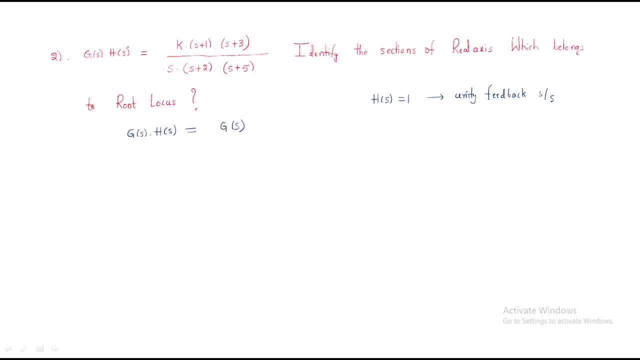 both are same, but to represents. to represents unity feedback system. he given like that, no problem at all. and the question is: g of s, h of s equal to k into s plus 1 s plus 3, by s into s plus 2 s plus 5. identify the sections. 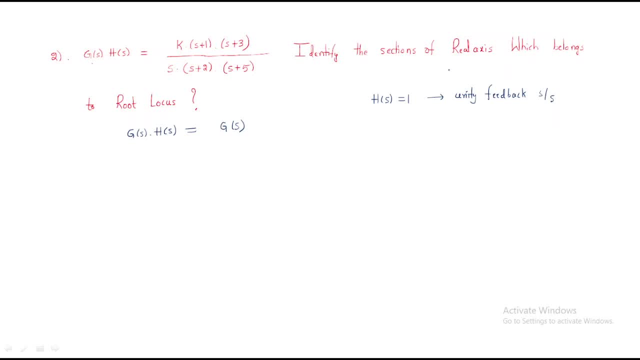 of real axis, real axis which belongs to root locus. so real axis, root locus. so so we have to follow the procedure. first, directly go for the root locus. yeah, first we will draw the diagram. just we will draw the diagram, this diagram, okay. so first identify the poles and zeros first. so identify the poles and zeros. 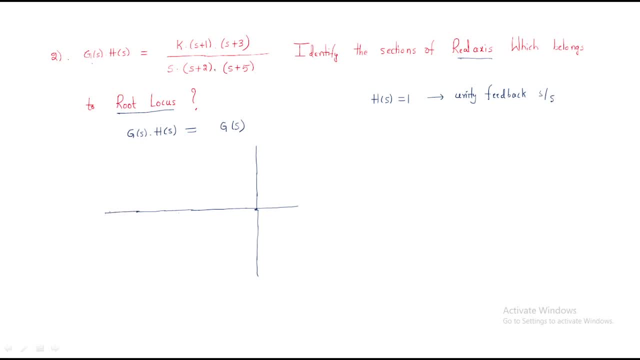 first. yeah, look at first. what are the poles? is there pole here? one pole is equal to zero, other pole is equal toマ, equal to 0, and the second pole is equal toiza, which is equal to 0.. minus two, another pose is s equal to minus three. so the terms which are in denominator is nothing. 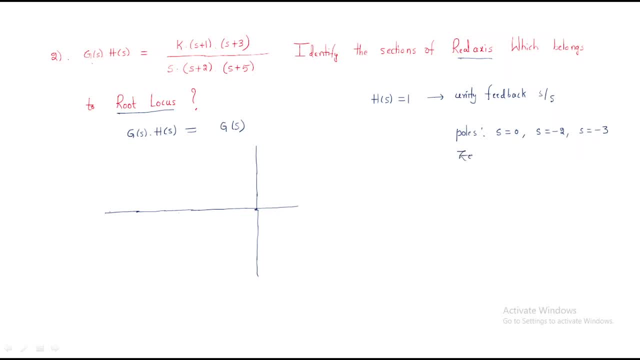 but the poles? what about zeros? zeros are s equal to minus one and s equal to minus. sorry, s equal minus five. this is, and this zero is s equal to minus three. these are the zeros. okay, from here just keep first. s equal to zero, always. pole. pole is represents with the, this symbol, and s equal to. 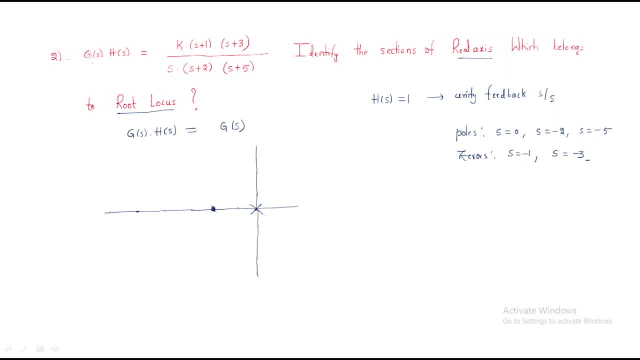 minus one is the zero. this is the s equal to minus one. take this value: s equal to zero and s equal to minus one. next is s equal minus two. so take it here: sum s equal to minus two and next s equal minus 3. minus 3 is the 0. again, so this is s equal minus 2 is actually pole, not 0, so 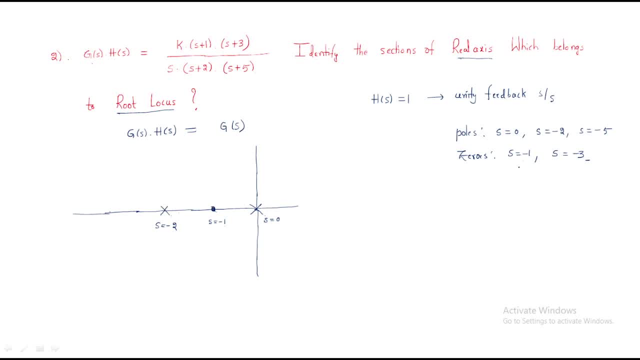 this is the pole, and s equal minus 3 is 0, s equal to minus 3 is 0 and 0- better to like the symbol. this is also a 0, so this is also a pole. this is also a 0 and we have s equal minus 5 is there. that is the pole. so we don't know where is the s. 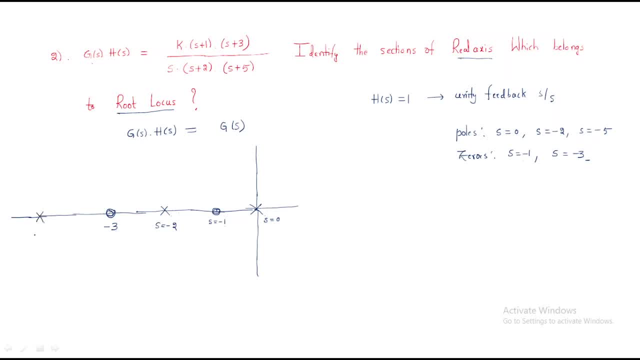 equal minus 5. just, I am taking s equal minus 5 is the pole s equal minus 5 is the pole. yeah, so I will be here. this is the s equal to minus 5 minus 5 is the pole. so these are the identification of poles and zeros. now 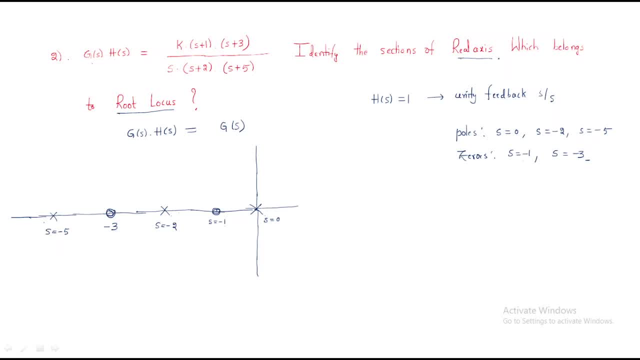 he is asking to find out real axis root locus. so way in the real axis where we have the root locus, right. so for that purpose, first. first, at this point, the right hand side combination of poles and zeros are zero. that's why we don't have any root locus here. but at this point, 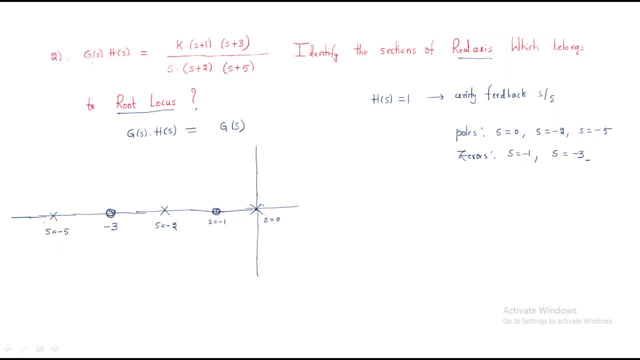 at this point, we have one pole, is there? the combination of poles and zeros is one. that's why we have the root locus at this point. we have the root locus here. and what about this point? this point: we have one pole and one zero. the combination is two. that's why we don't have any root locus. 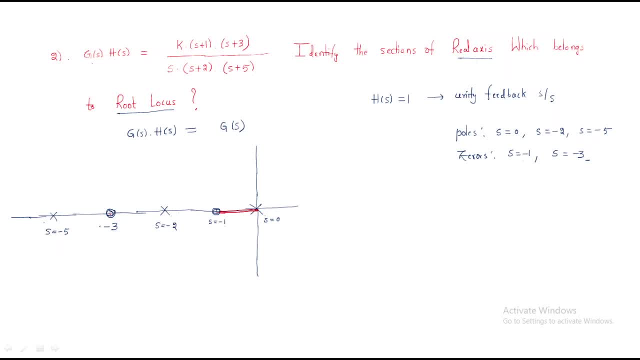 at right side for this, but at this, at this s equal to minus three s equal to minus three here. one, two, three, three are there, though. that's why we have the. we have three, yeah, and we have the. root locus is there, and root locus is available here. and the next. 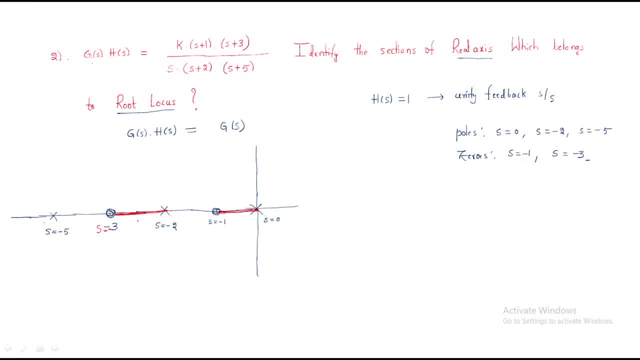 point here. the next point s equal to minus 5 for this point. at this point we have one, two, three, four, so we don't have anything. we don't have anything. so here the most important point is there. so always the root locus is like this: it starts from pole and end with the zero. so look at here here s 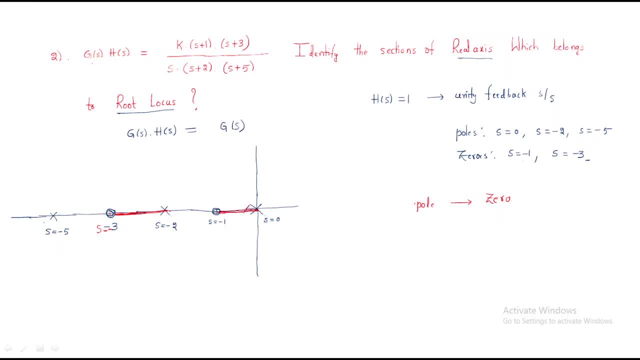 equal to zero is there s equal minus one there. so root locus is: starts from zero and end with starts from pole and end with zero. this point to this point, that means this point dc gain is zero. at this point dc gain is infinite. like that. and if you observe here: 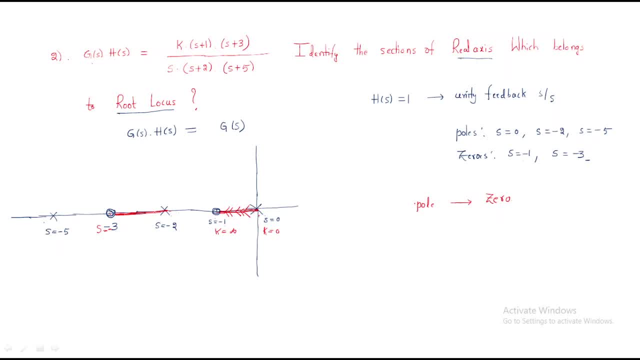 and we have the one pole and one zero at s equal minus two starts from root locus and end. root locus is zero. that is, k equal to zero here and k equal to infinite here. and at this point we have the pole here we don't have. we don't have zero here. so that's why 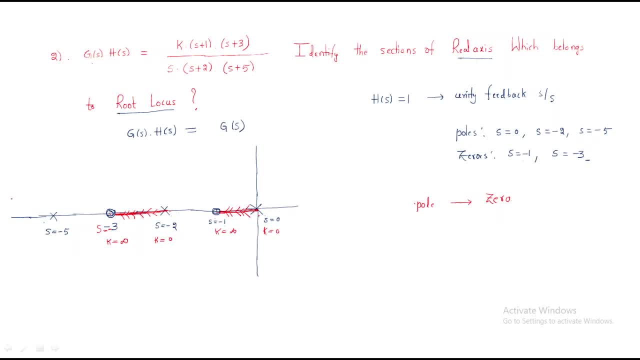 we are assuming zero is somewhere infinite. we don't know, but somewhere infinite we have the zero and from this pole the root locus will be extended like this. extended like this, okay, so the losses will be number: number of root locus branches here. so that's why observe here: 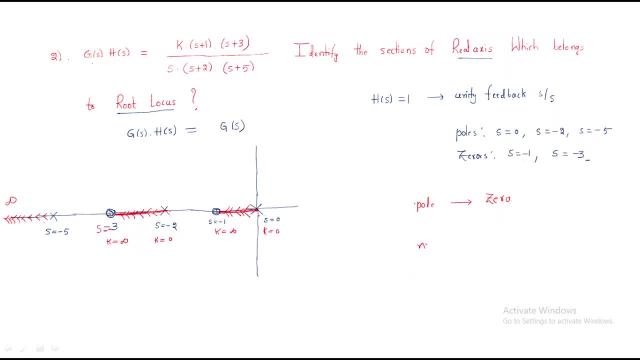 the number of root locus branches. here number of the number of root locus branches will be equal to which is the major. so here zeros are two, only poles are three. that's why number of poles, that is the three. look at here: this is the root locus one, and this is the root locus two, and this is the root locus three. so we have three root locus.